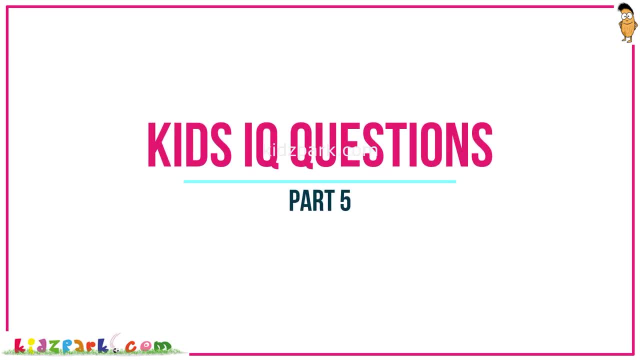 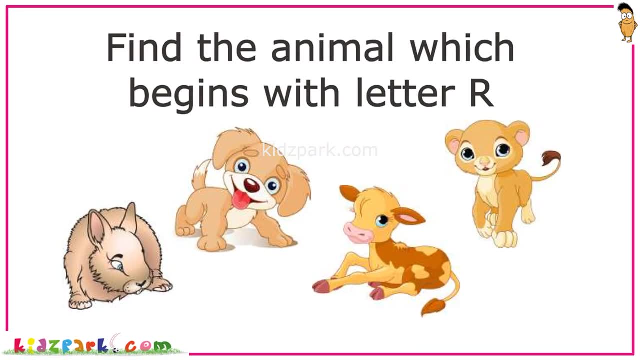 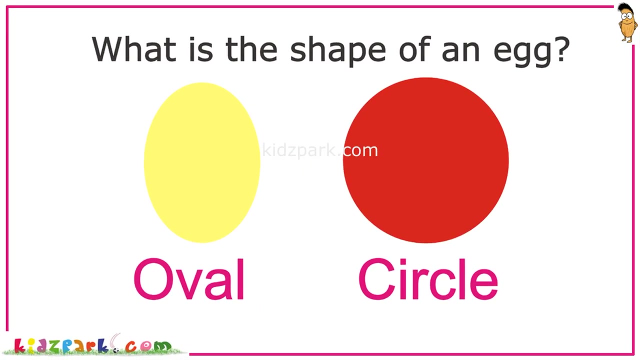 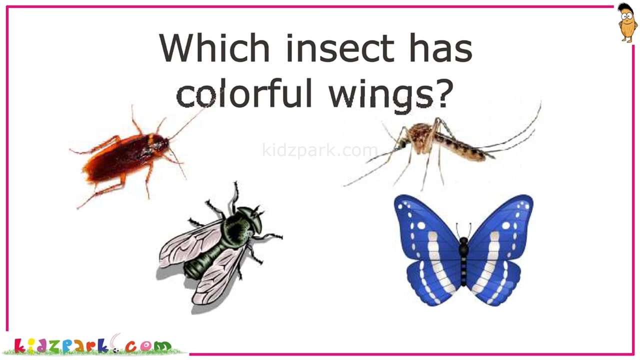 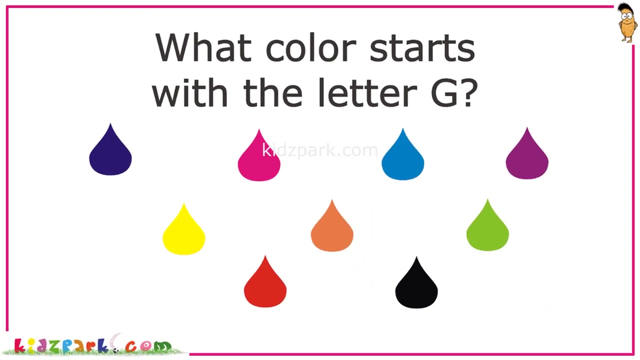 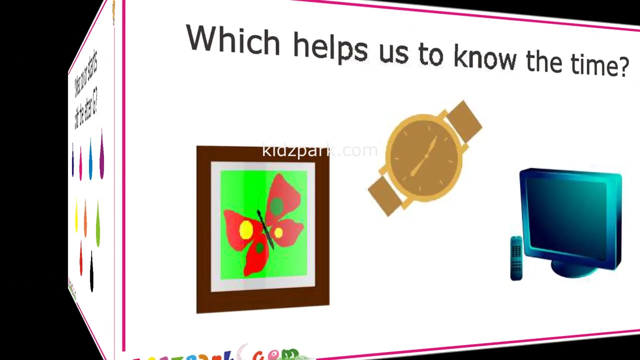 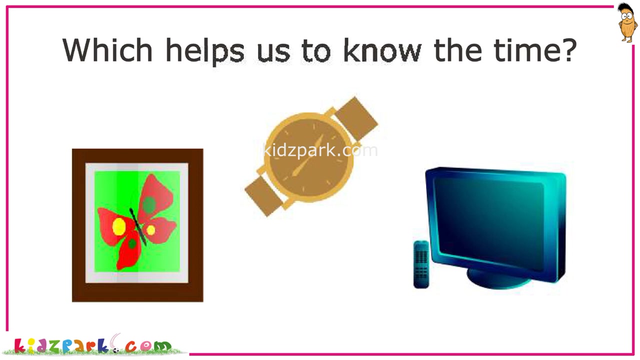 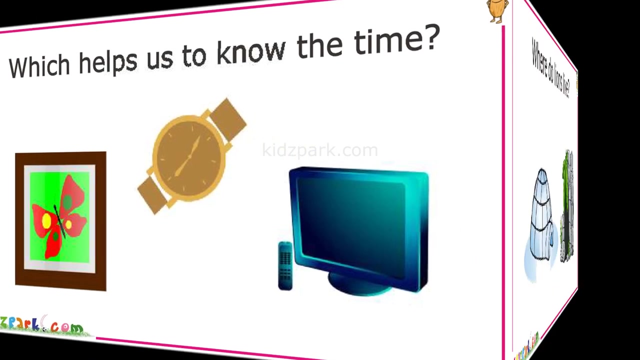 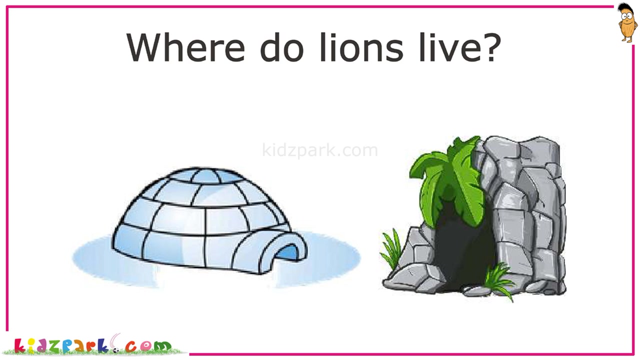 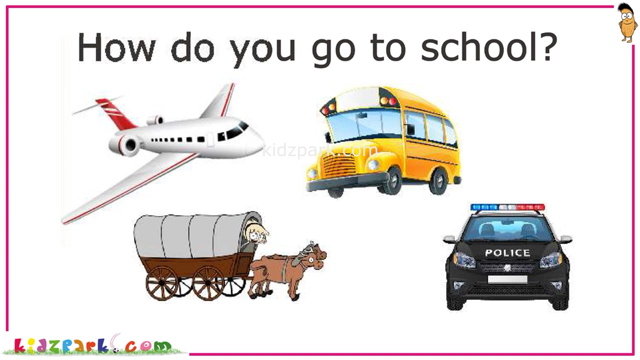 Find the animal which begins with letter R. What is the shape of an egg? Which insect has colorful wings? What color starts with the letter G, Which helps us to know the time? Where do we start? Where do lions live? How do you go to school? 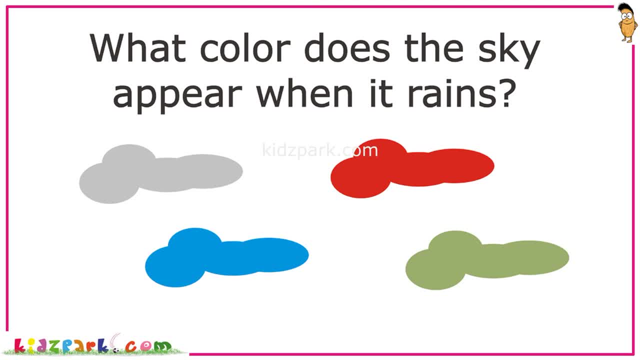 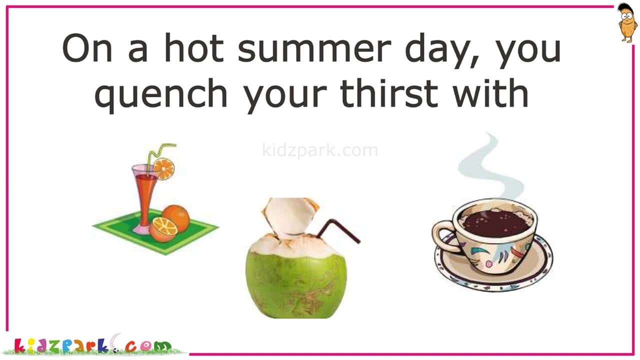 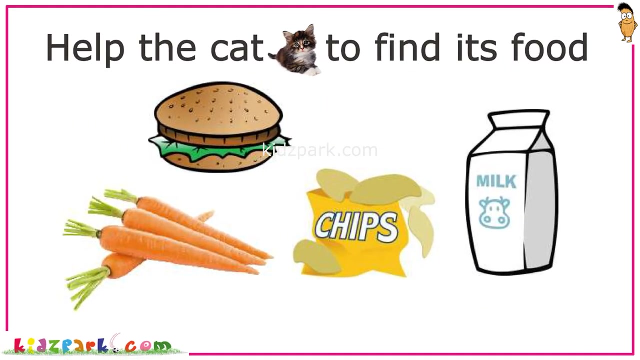 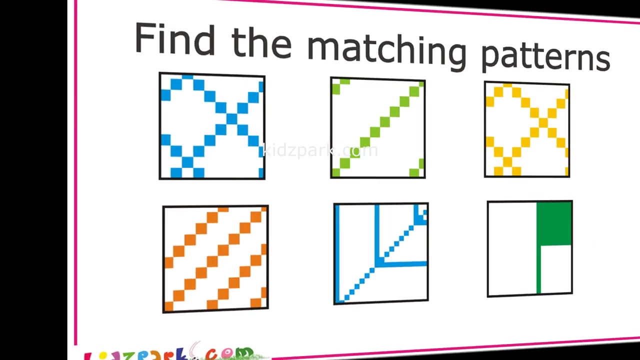 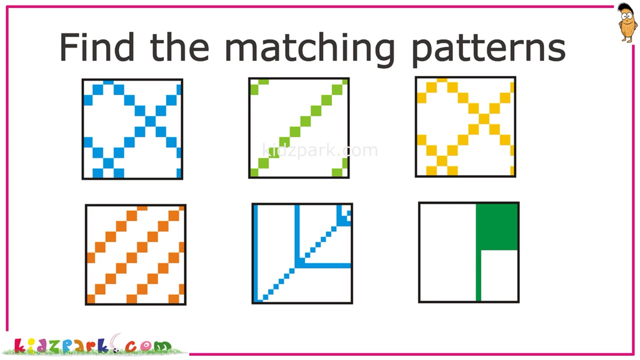 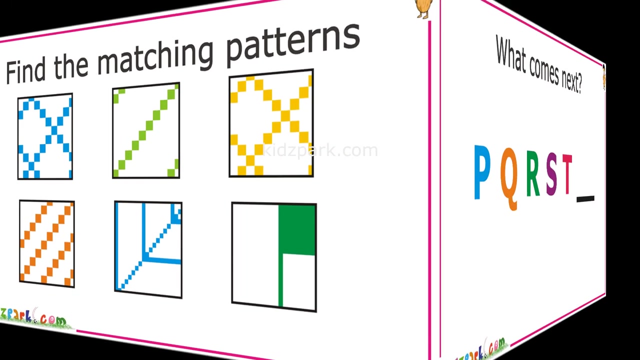 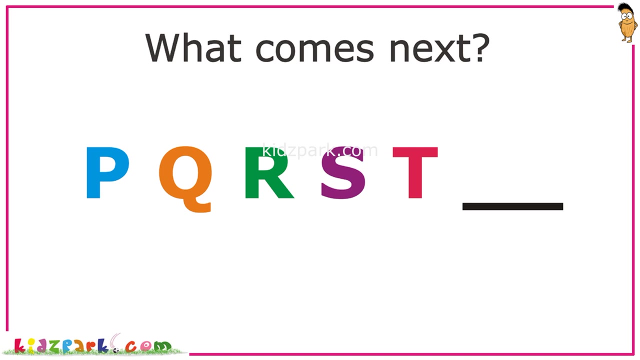 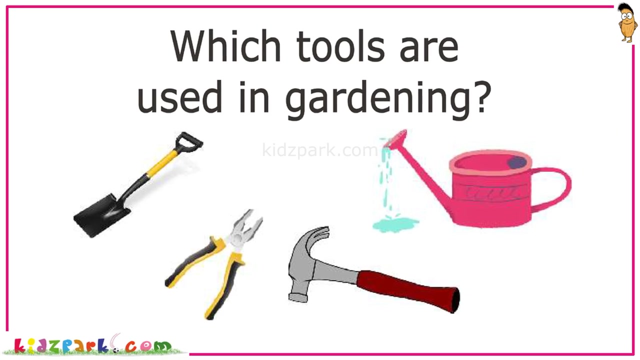 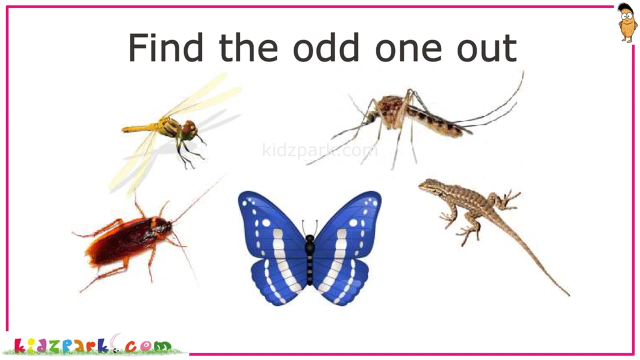 What color does the sky appear when it rains? On a hot summer day, you quench your thirst with. help the cat to find its food. Find the matching patterns. What comes next? Which tools are used in gardening? Find the odd one out. 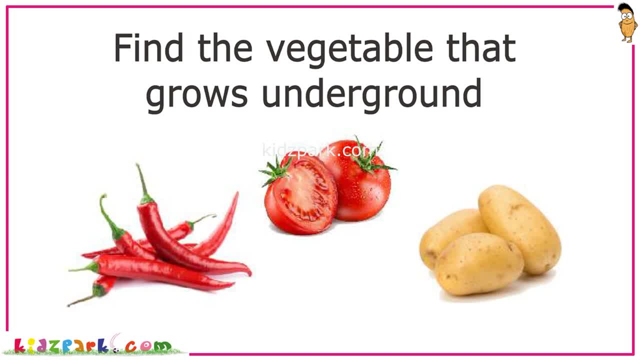 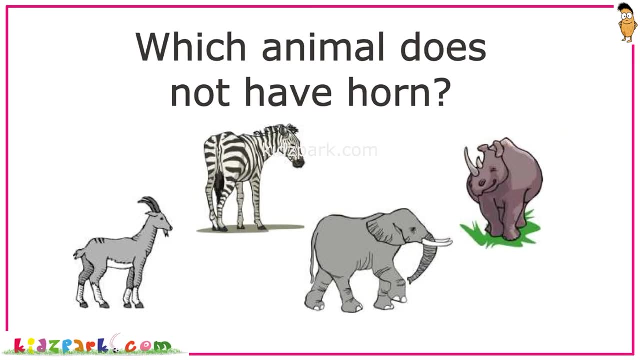 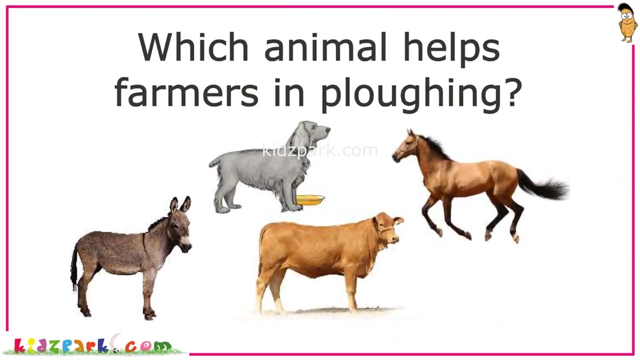 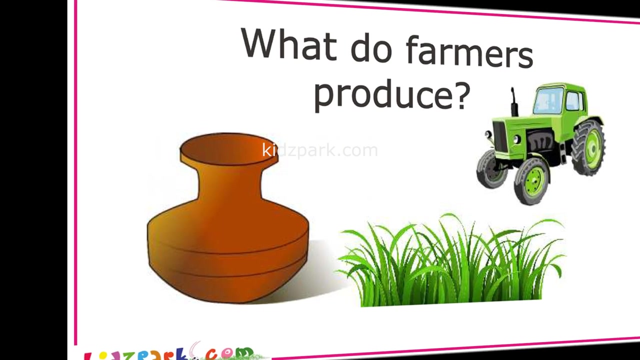 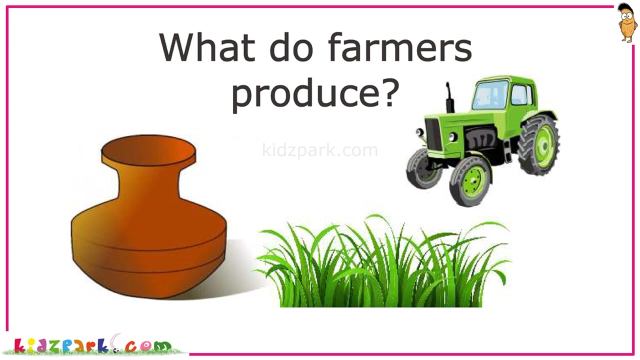 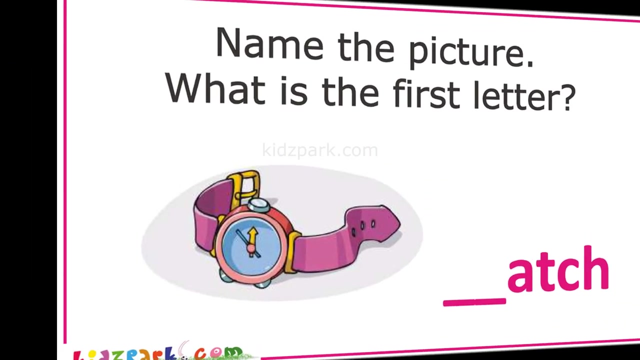 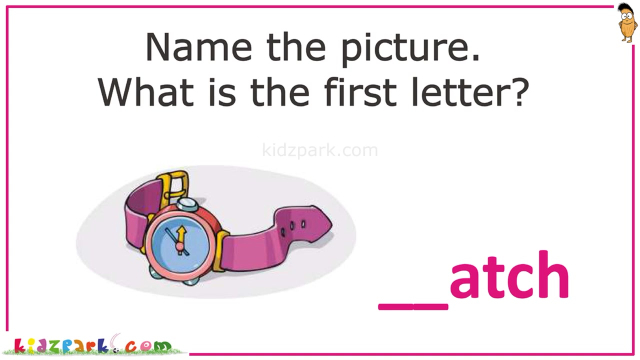 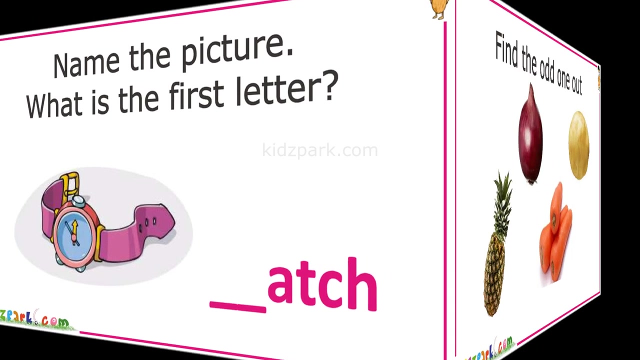 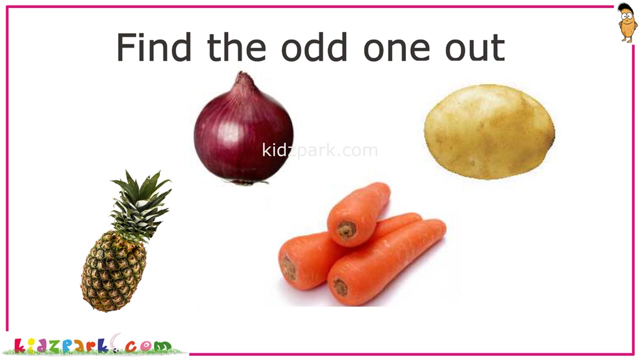 Find the vegetable that grows underground. Which animal does not have horn? Which animal helps farmers in plowing? What do farmers produce? Name the picture. What is the first letter? Find the odd one out. Which animal does not have horns?